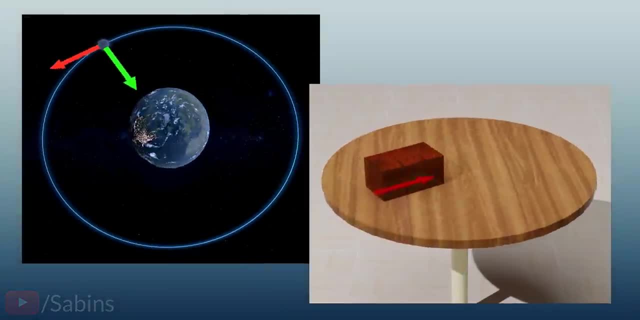 This means, if the time interval of applied force is significantly smaller, you will get a more perfect circle. This means, if the time interval of applied force is significantly smaller, you will be able to move in a circle. This means, if the time interval of applied force is significantly smaller, you will be. 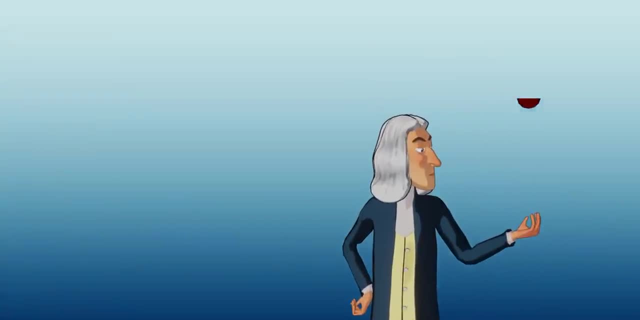 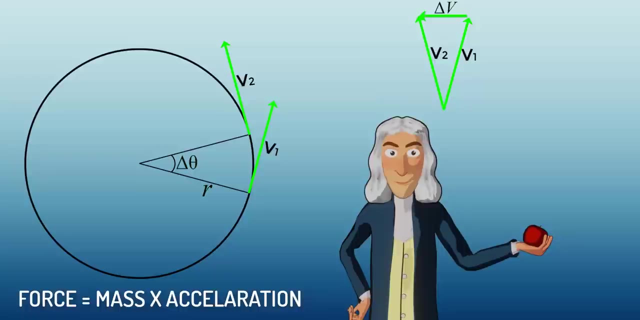 able to move in a circle To get the value of the centripetal force. we should approach the problem analytically and start with the way Sir Isaac Newton defined force. However, there's no fun in an analytical derivation, so we'll animate this method. 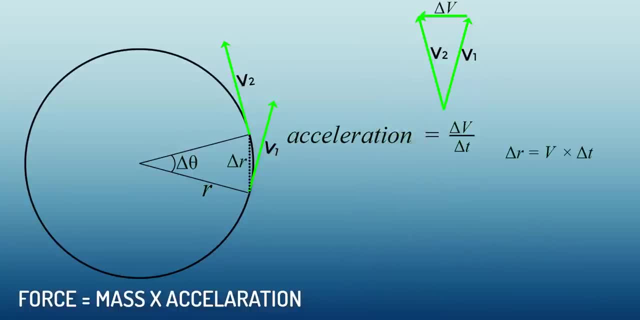 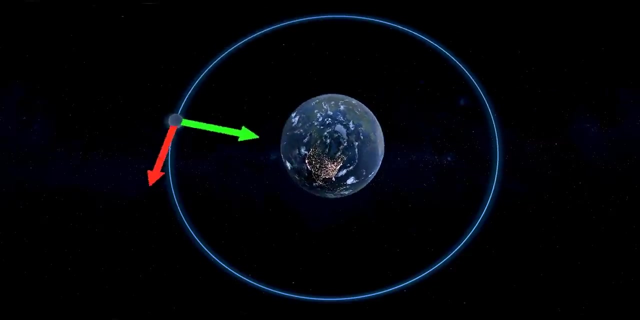 The conceptual understanding we already developed will really help you in science and engineering. Once again, it is clear from this equation that the lesser the radius of the circle, the more centripetal force will be needed When the Moon revolves around the Earth. the gravitational force acting between the Moon 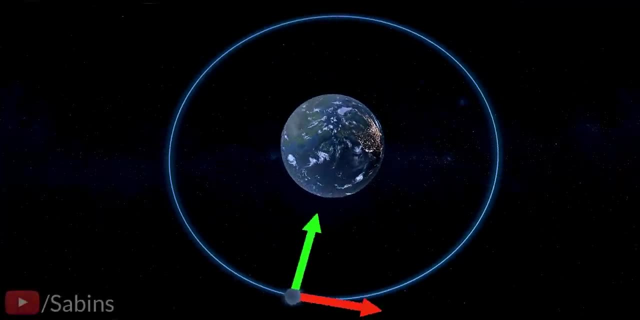 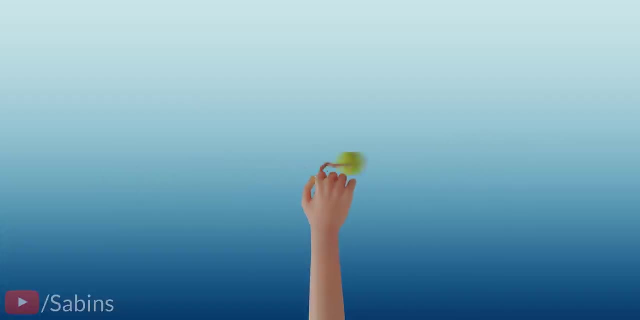 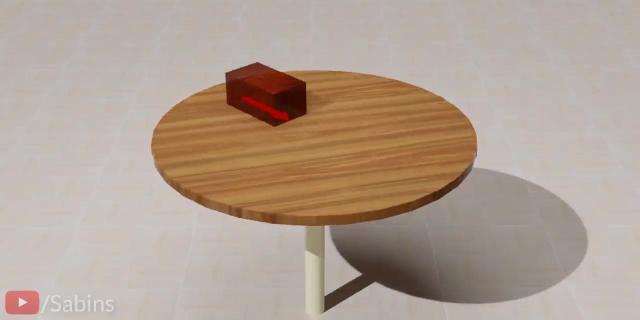 and the Earth provides the necessary centripetal force. Similarly, when you rotate an object attached to a string, the tension in the string provides the required centripetal force. Consider this spinning wooden block. The frictional force between the block and floor lends the necessary centripetal force. 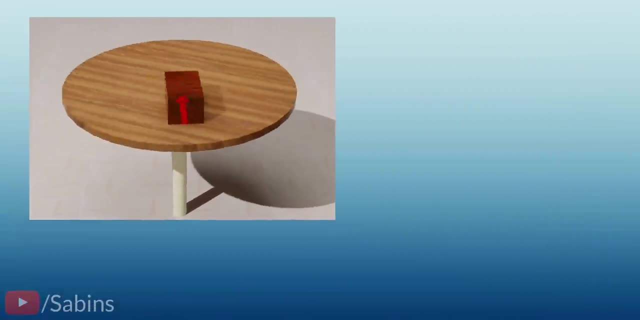 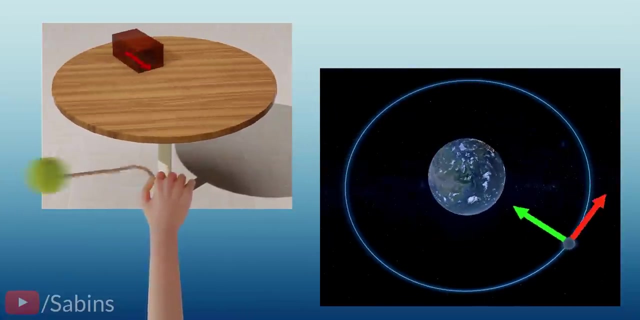 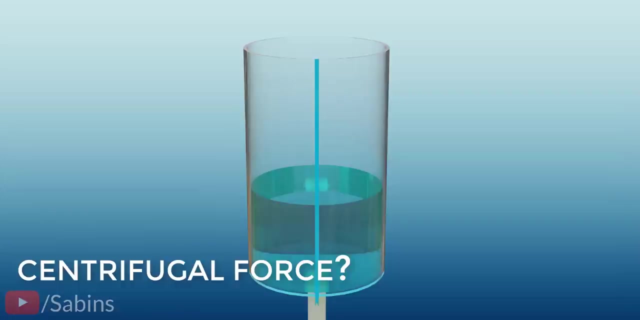 In short, centripetal force should be supplied by some external source, such as gravitation, tension, friction, etc. Now that we've learned the concept of centripetal force, the big question is: what is centrifugal force? Consider these examples. 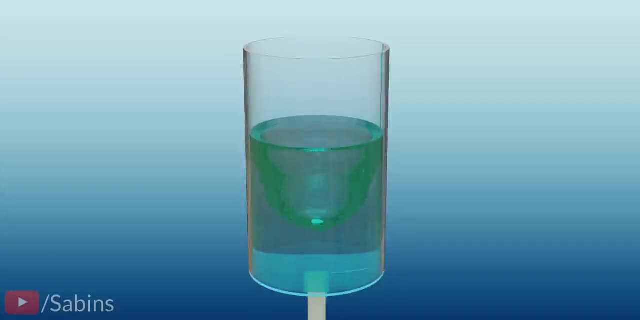 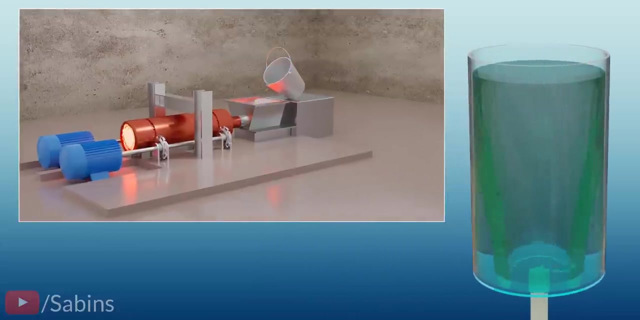 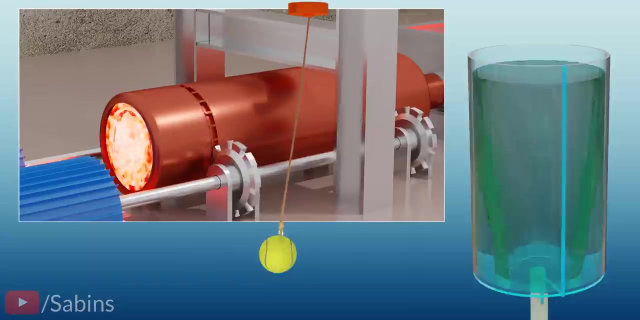 When fluid spins in a beaker, as the speed of the beaker increases, the fluid flows outward. Similarly, in this centrifugal casting process, the molten metal always moves. This moves to the outer wall. As you increase the speed of this suspended ball, the ball also travels outward. 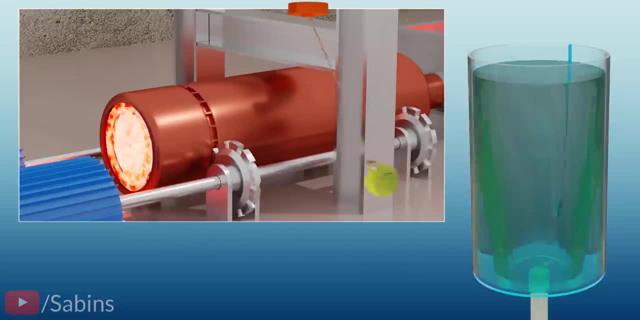 Is there any force called a centrifugal force which is acting radially outward on a rotating object to move it outward? Scientifically speaking, there is no such force as a centrifugal force. It's a pseudo-force. A rotating object always needs a force which is radially inward. 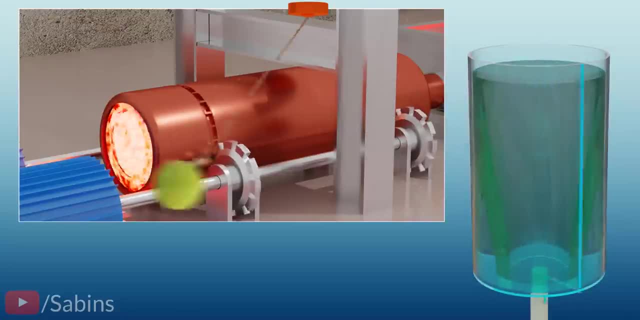 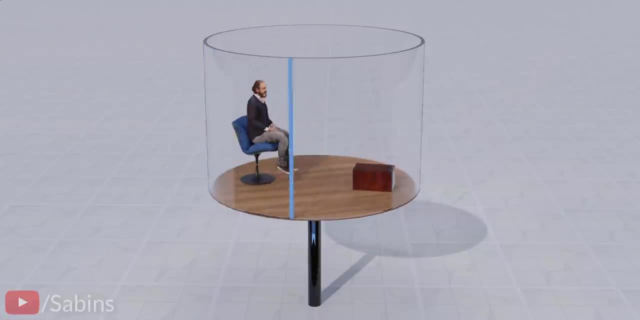 Centrifugal force is needed. in fact, Centrifugal force is needed in physics only when you analyze the problem rotating along with the object. In this example, since the observer is sitting inside a rotating cabin, the observer has to add a centrifugal force to analyze the problem. 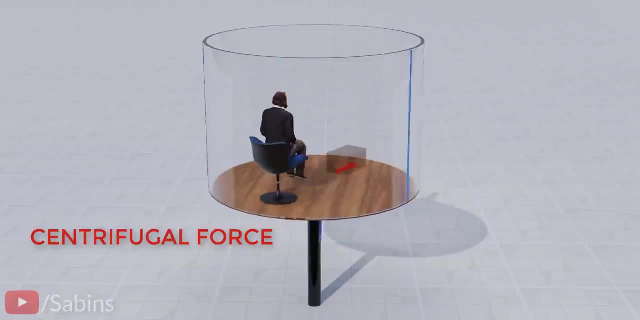 It's a pseudo-force added to convert a non-inertial frame of reference to an inertial frame of reference. If the observer is on the ground, there is no need to use such a force. Now let's analyze the previous examples using the concept of centrifugal force. 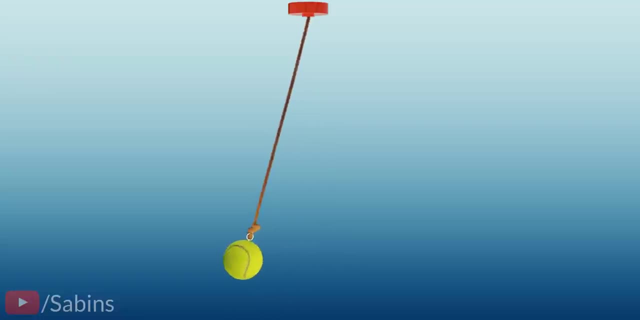 The first example is a centrifugal force. The ball rotated using the centrifugal force. By αυτing thethis expression, we make sense of the process of the ball not moving away. Using the concept of centrifugal force we have developed 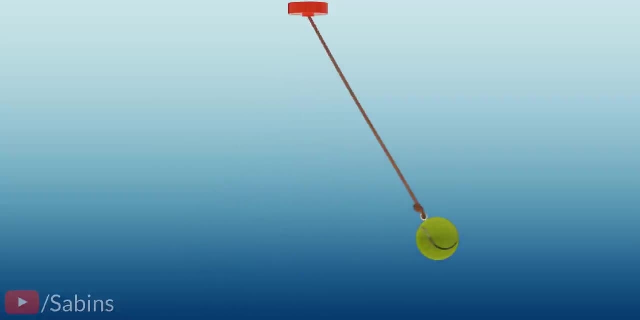 As you rotate the ball, faster it moves away. The ball needs a redefugal force. The tension of the rope, more specifically the horizontal component of its tension, provides that force. The tension on the ball has one more responsibility. The vertical component of the tension has to balance the weight of the ball. 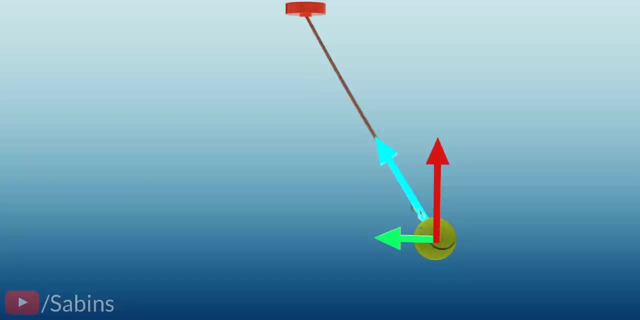 The vertical component of the tension has to balance the weight of the ball. We have now come to the last part of this way. Logically, as the ball rotates faster, the rope's tension should increase to support the tension which has been predicted. 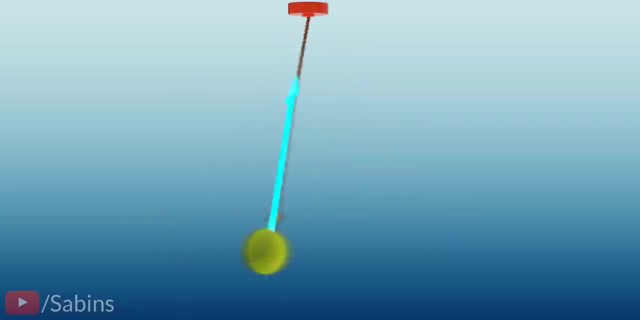 But āof effect Out of one step, the sufficient centripetal force. However, the weight of the ball does not increase, which means that in order to keep the vertical component of the tension the same, the angle has to increase. 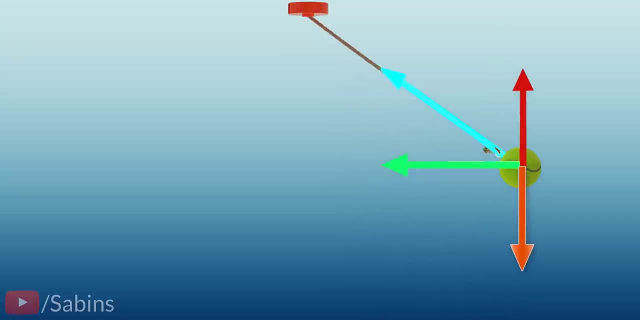 like this. This is the reason why the ball moves away as you rotate it faster. The case of the rotating fluid is slightly different. Here again, each fluid particle requires a particular amount of centripetal force to maintain the circular motion. The pressure difference caused by the water level's height disparity. 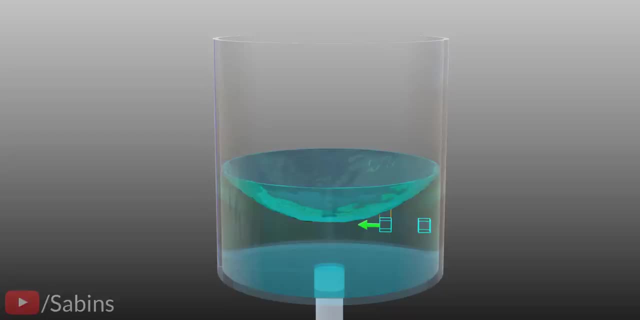 generates that centripetal force. The fluid particles at the outer radius obviously need more centripetal force. To satisfy this increasing centripetal force requirement, the fluid surface has to form a curved shape rather than a straight line. Here each particle demands more centripetal force. 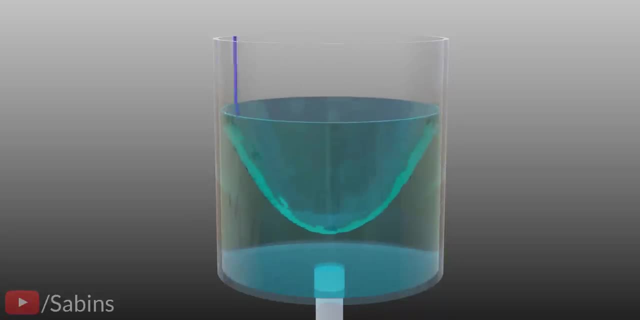 or more pressure difference across the particle. Therefore, the water surface curves more than in the previous case Or you feel like the water is going outward. It's better to avoid using centrifugal force in your scientific or engineering analyses, because it's a pseudo-force used only in some special cases.